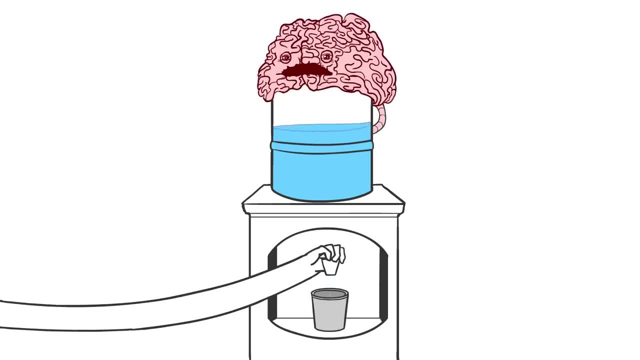 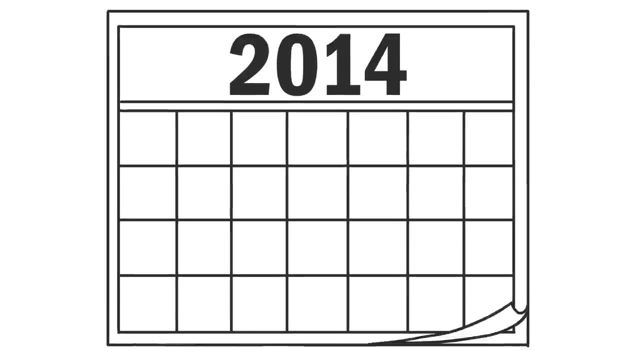 represents my accumulated knowledge nor my passion for architecture. It merely serves as a reminder of how many years I can endure hating myself. True, it has been almost 10 years since I graduated, so it's natural that I forgot a lot of what I learned. but even at the year of 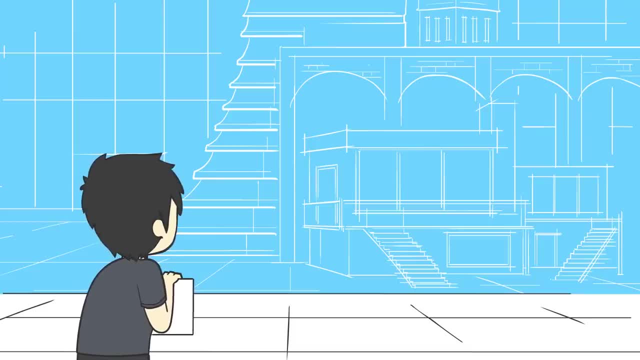 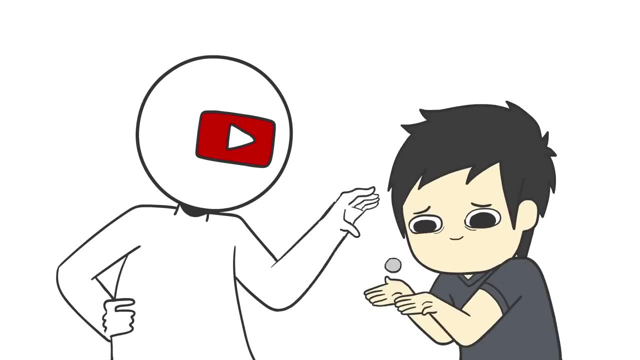 I didn't really have confidence with my knowledge in pursuing the field When I chose to full admit to YouTube and content creation. I naively thought to myself: if I totally bomb this and I make like 10 cents a month, at least I have architecture to fall back on. But really it was more like 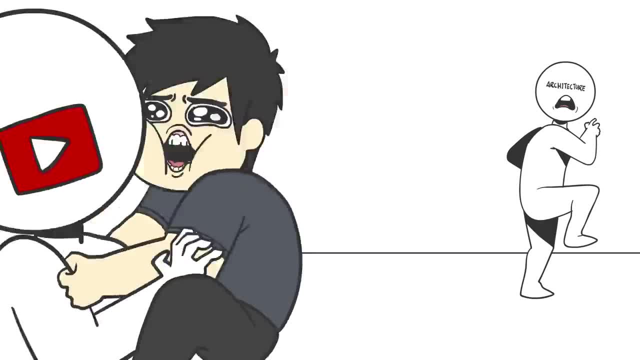 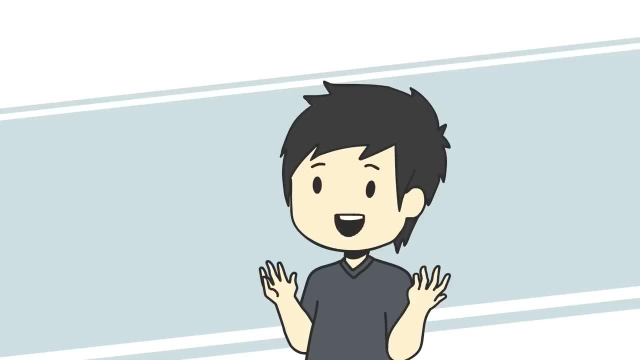 please let this work. I don't want to do architecture. I hate it. I want to make dumb animations, Please. Architecture wasn't really plan B, It was more like plan L. So when I say I truly appreciate your support of my work and allowing me to self-sustain from my videos, 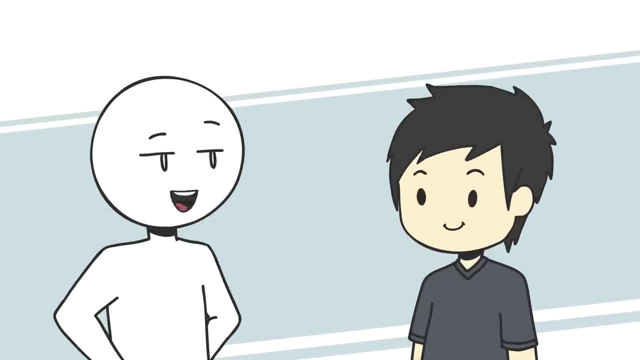 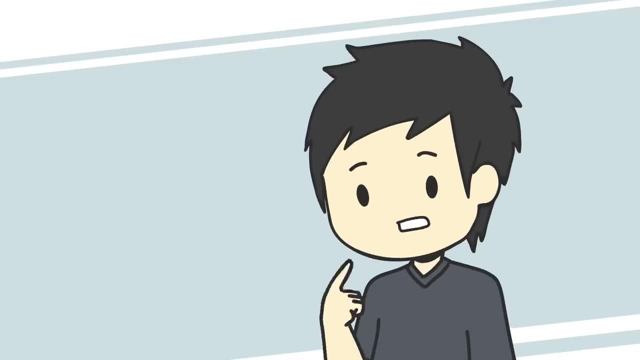 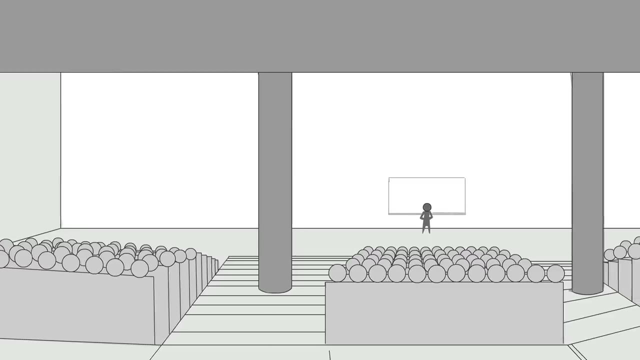 I really mean it. Thank you all. That's really awesome, Dom Thanks. So how much did you retain from architecture school? Oh, let's see Um one. well, I cried at least 17 times. I remember one of the first lectures we had, our prof. 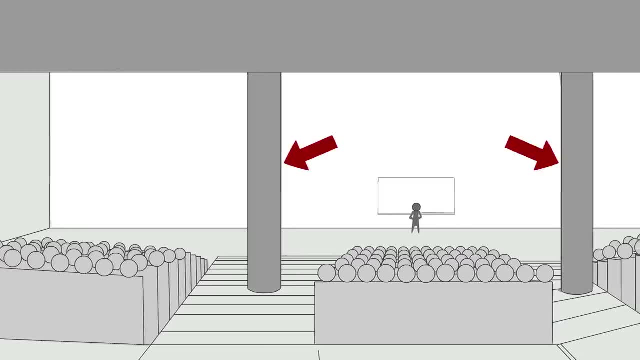 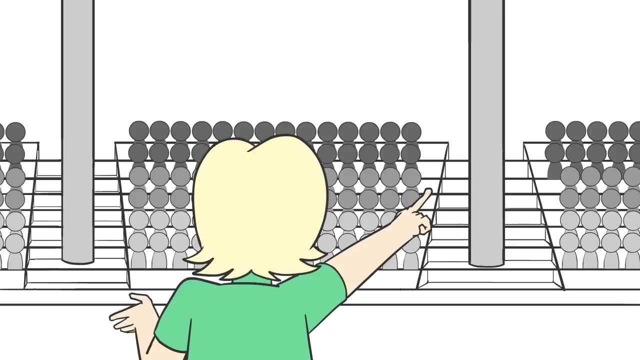 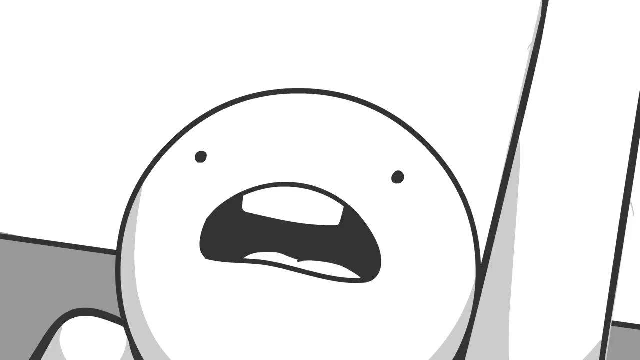 shat on all of us for not knowing what this structural element is properly called. Anyone know what that is right there in the middle of the room? What is that called? Yes, A post- Nope. A pillar: Nope. A beam, A vertical beam- Nope. One more try or I feed my shoe to one of you. 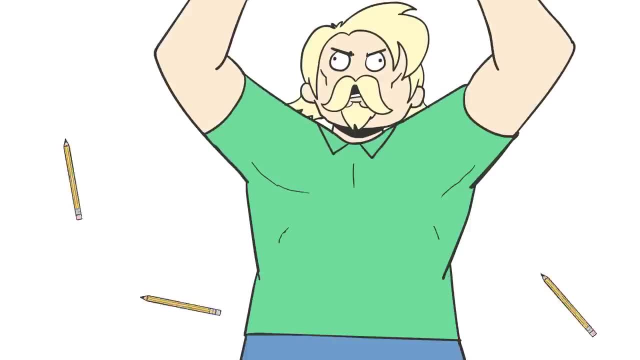 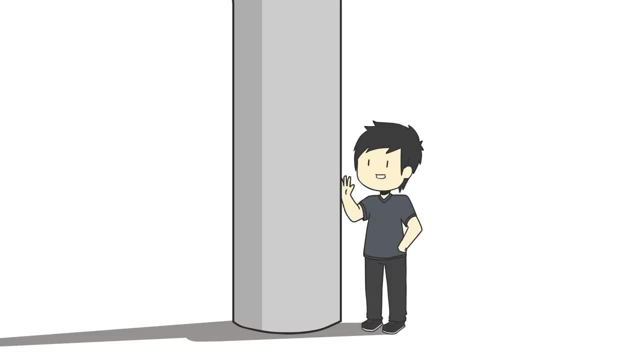 A structural vertical beam, A column. It's called a column. How do you guys not know this? You're in first year, God. So for the rest of my life, due to being ridiculed, I will know to call this a column Boy. I'm sure glad my tuition paid for someone to make fun of me for going into 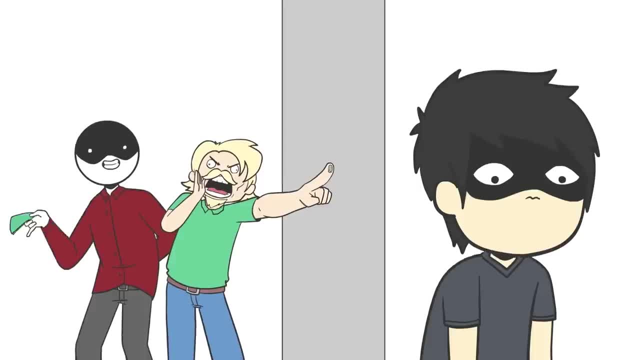 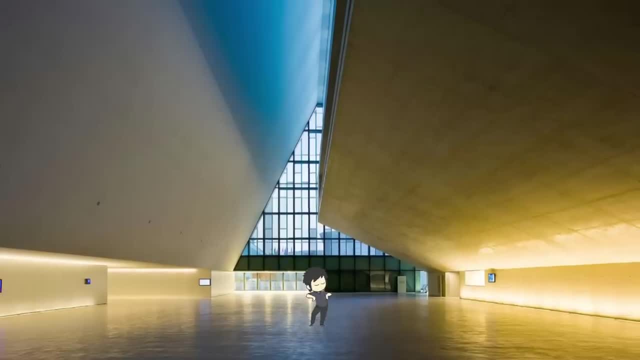 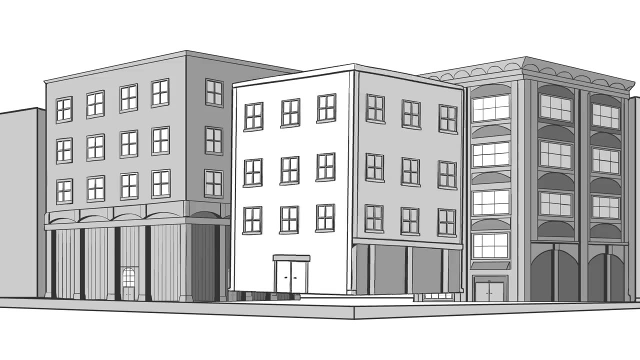 a program to learn about things I wasn't knowledgeable about. The biggest lesson I've learned in what makes a good building design is: form follows function. The nature of architecture is to design based on the human experience and how people interact with the space. The overall shape of the building should 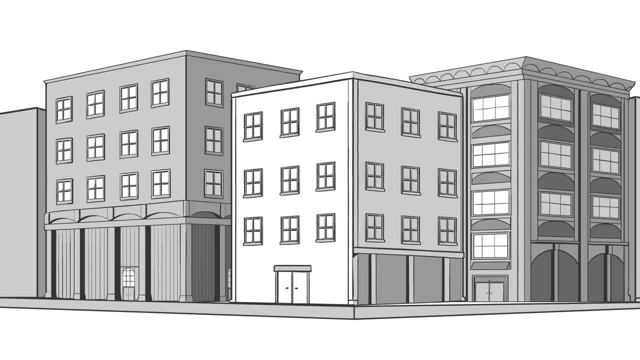 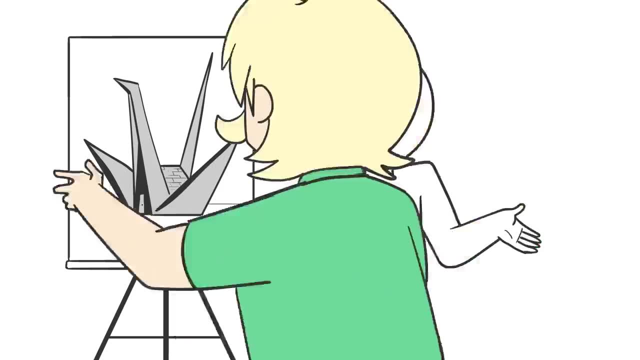 be directly corresponding to the intended function or purpose of the spaces within it. If you design a building shaped like an origami paper crane and presented it to a professor for a critique, they will calmly tell you it is garbage and then spit on your grave because 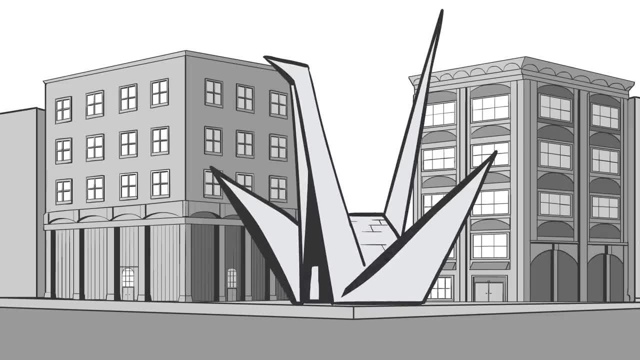 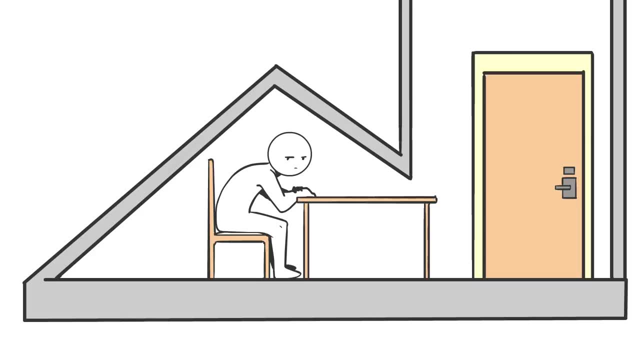 you are now dead to them. Even though seeing a paper crane building might seem cool and instagrammable, when you think about it, it likely fails as a building. You've got awkward corners everywhere, making awkward rooms for people to fit into, which means 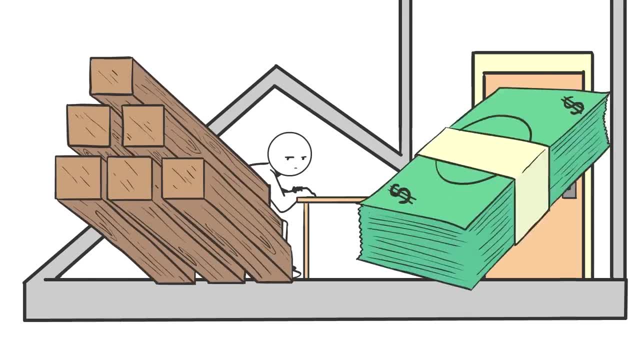 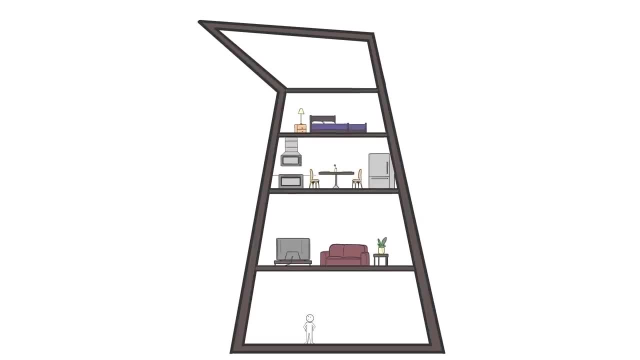 a bunch of wasted space and wasted construction materials and costs. and what is even going on up here? Is it just a tall empty space, or are there awkwardly shaped single rooms that shrink every story until you get to the sniper tower? How do you even get up there? 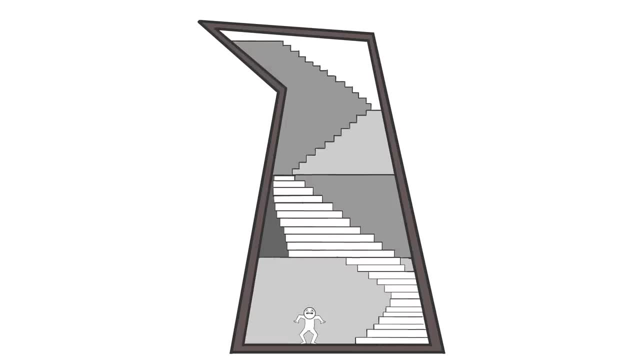 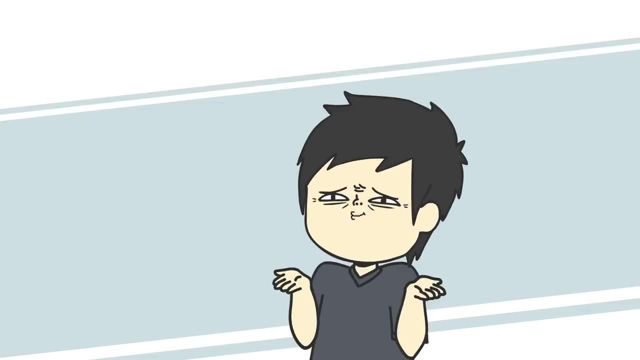 Standard elevators don't move diagonally and stairs aren't gonna fit nicely without the engineers wanting to put a bounty on your head for this complicated design. Simply put, if it's annoying to build, it's probably a bad design. While a paper crane may be used as inspiration for a design, there is much. 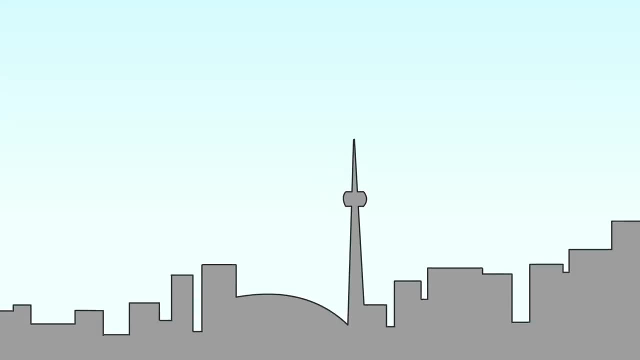 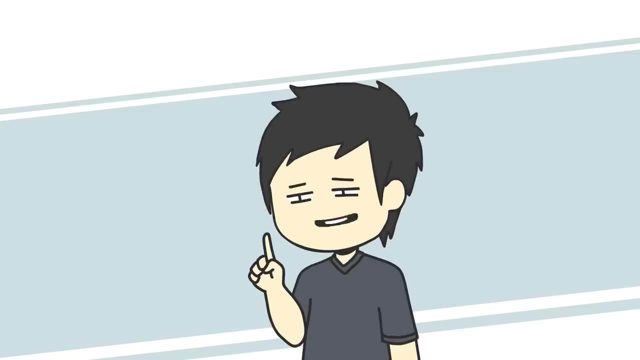 more to architecture than just cool visual concepts. There is this museum in Toronto called the Royal Ontario Museum, the ROM, and all of my professors, collectively and unanimously, shit on the ROM every chance they get. It looks like this, and you might. 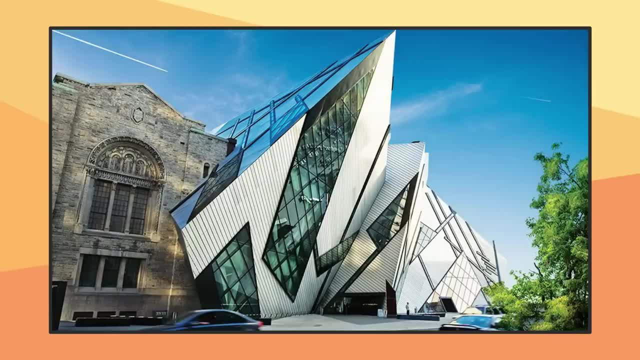 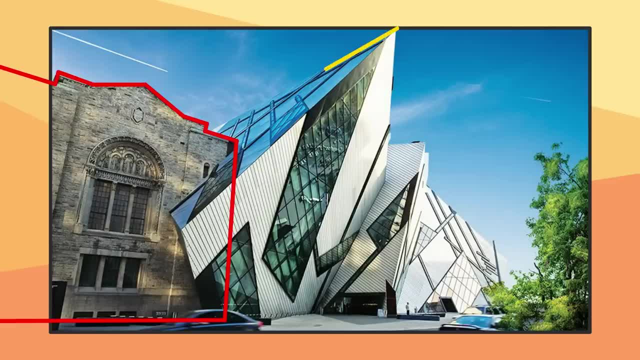 It's got some very odd details. It's got some very odd details. It's got some very unnatural shapes and it's interesting how it superimposes on the surrounding structures to elaborate the distinction between the old and the new. It stands out Very touristy, But that's. 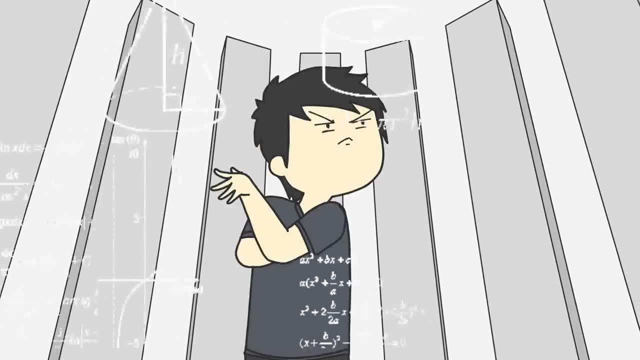 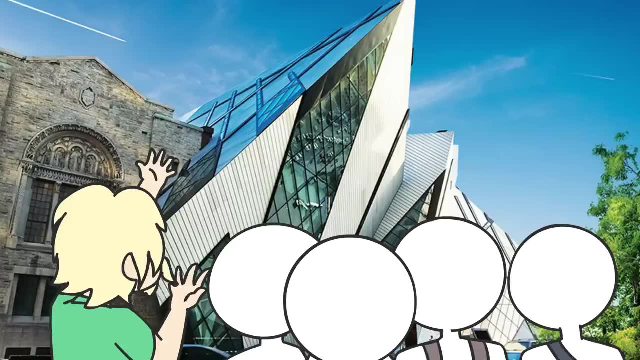 all it did Stood out. Once you go through architecture school, you never look at buildings the same way ever again. You know how much my profs hated the ROM. They took us on a field trip to the ROM to shit on its design during the tour. Wow, look at all these awkward. 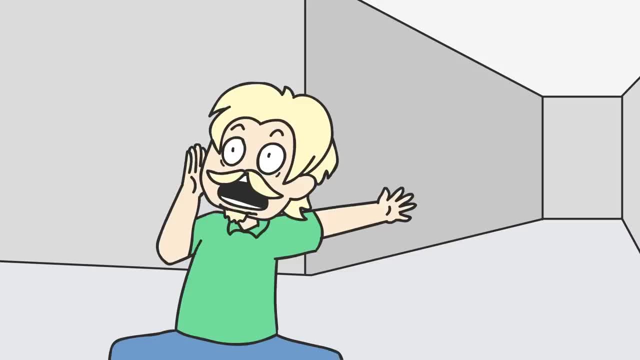 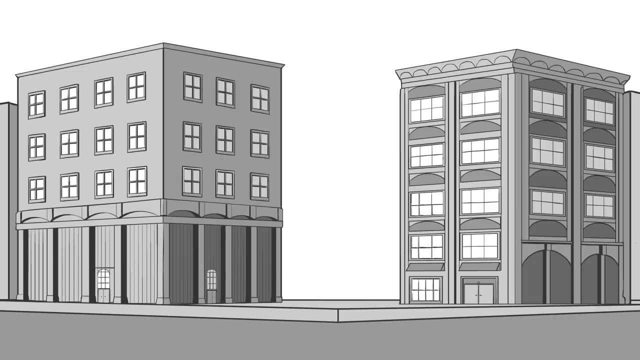 corners. Wow, look at all this wasted space. Wow, look at this useless hallway that leads to a dead end. Wow, wow, wow. They were brutal, but they were right. Some people might feel like square and rectilinearly designed buildings are basic and boring, but 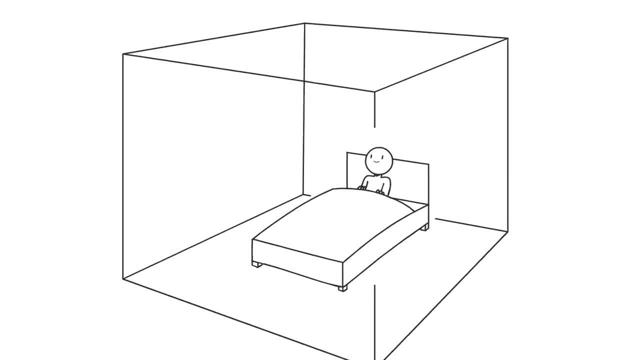 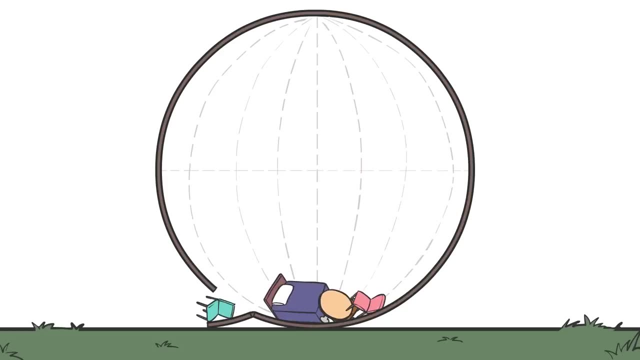 really, it's those kinds of spaces that we usually feel the most comfortable in. What the hell are you gonna do with a spherical room? Where does your door go? How are you gonna arrange your furniture to fit without having to customize them? Are you gonna have 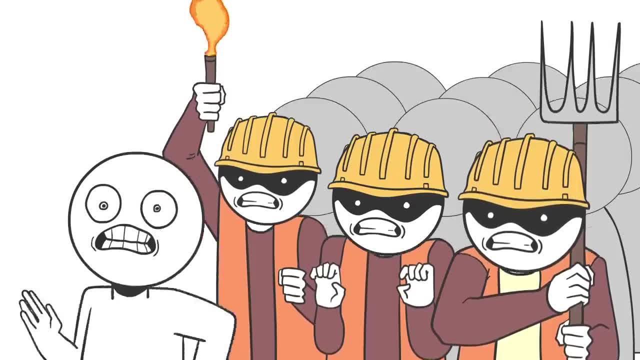 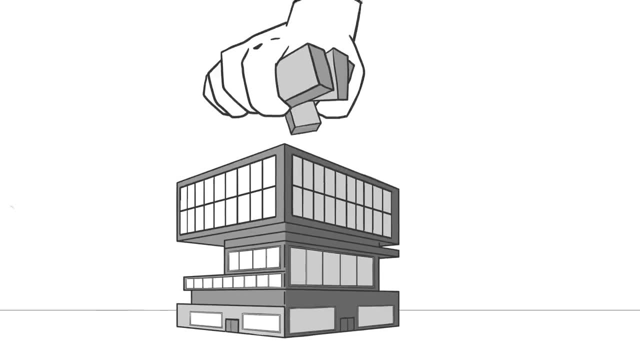 curved glass windows. Again, the engineers and construction workers will have your head on a pike. Remember, form follows function. You don't think of how a building will look and then somehow force-cram the necessary rooms inside to fit. You keep in mind your overall space. 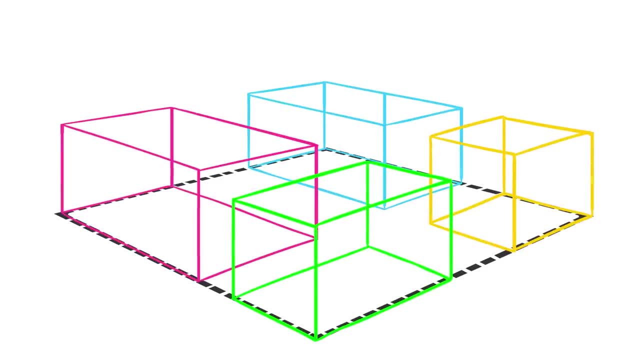 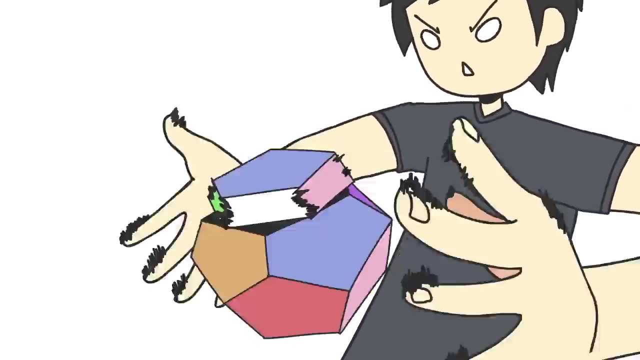 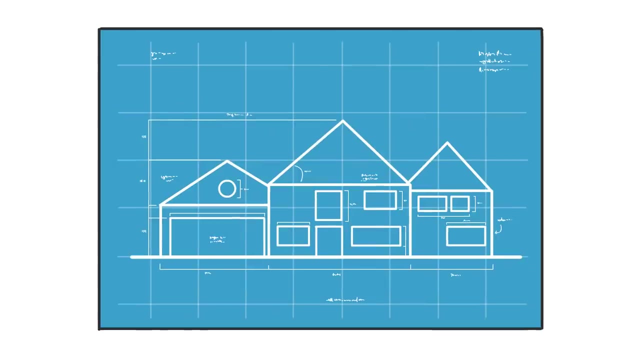 constrictions, of course, but you have to design from the inside and eventually the outside will take its form, And finding the optimal arrangements in correspondence to interesting forms is what sets aside the good architects from the paper crane designers. Some other bits of things I learned. We never called these blueprints, They're just called. 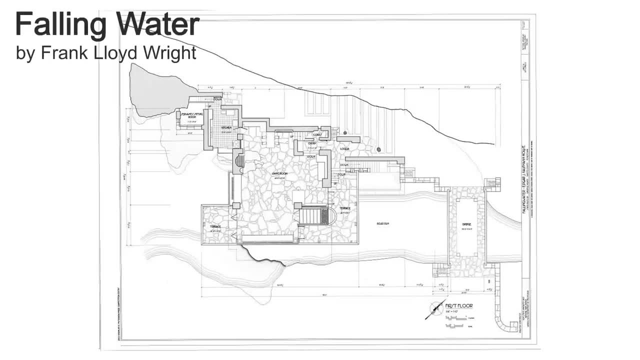 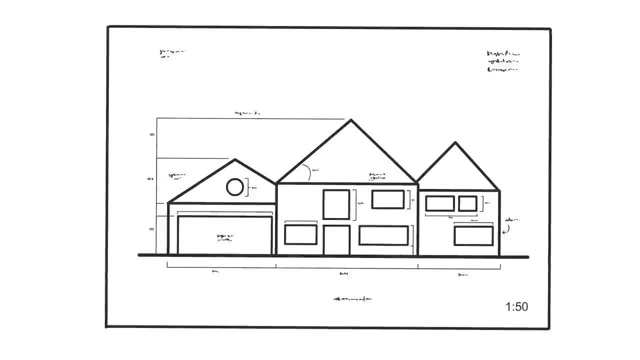 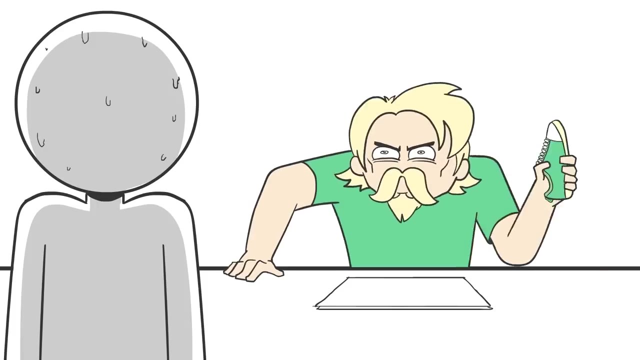 architectural designs. These are the drawings made up of plans, sections, views of the spaces as if you cut through it, and elevations Always include standard scales. when showing drawings, 1 to 73 is not typically a scale. people understand This part of the. 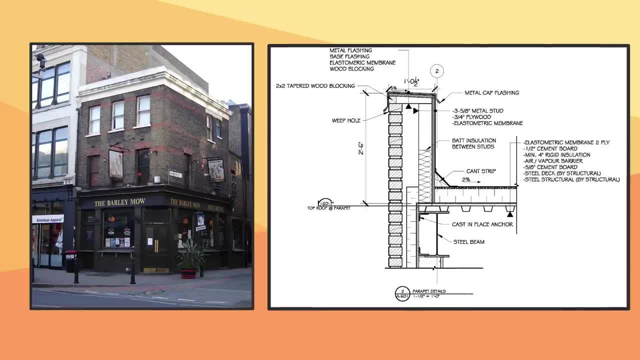 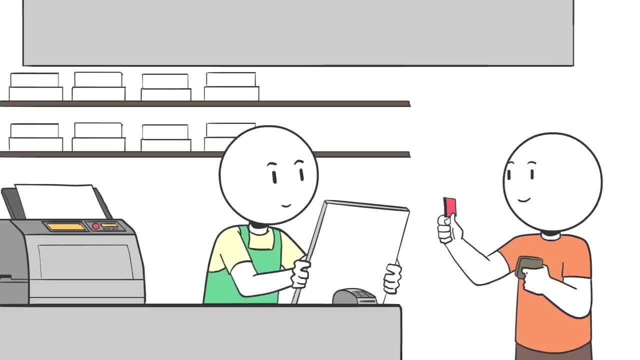 roof of a building is called a parapet, and it was really annoying to draw in cross-section. Either you drew your drawings on a presentation board by hand or you did it on a computer and spent $90 to print it. Starving artists. 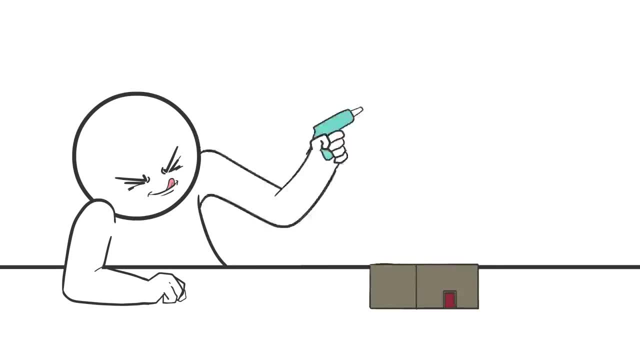 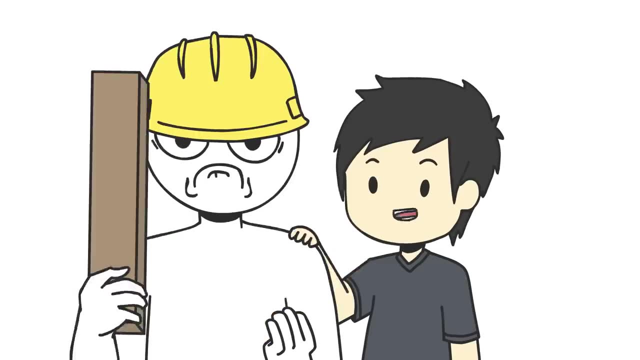 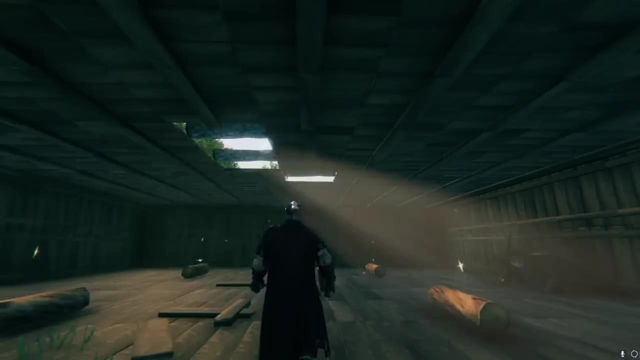 Starving architecture students Get along. Avoid using glue gun for your models. It doesn't dry nicely and sometimes leaves those spider-web glue bits, As I've mentioned before. keep the engineers in mind. They have to make your design stand. If you think a 20 by 20 meter room can hold up without any columns, enjoy having your. 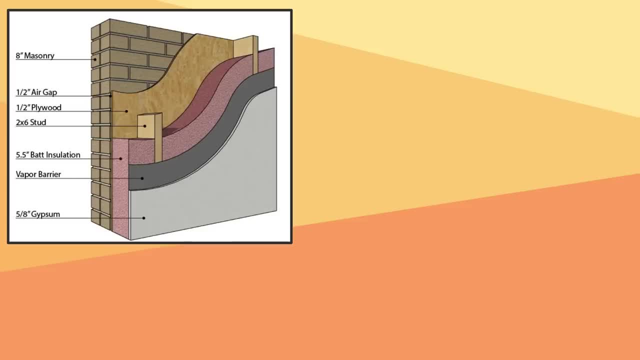 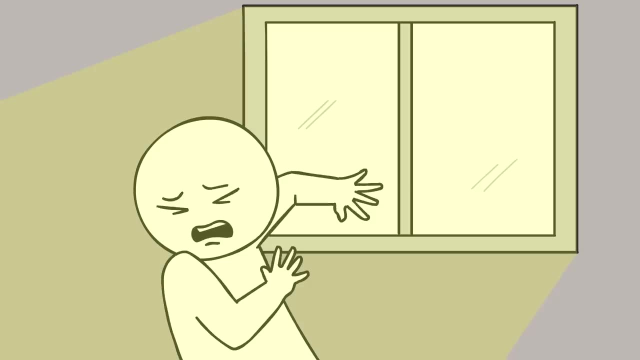 ceilings collapse. Exterior walls are much thicker than you think because of insulation. Flooring is much thicker than you think because of HVAC. East and west facing windows give harsh lighting because of insulation. If you don't have a good ceiling, you might want to fix some of the parts. 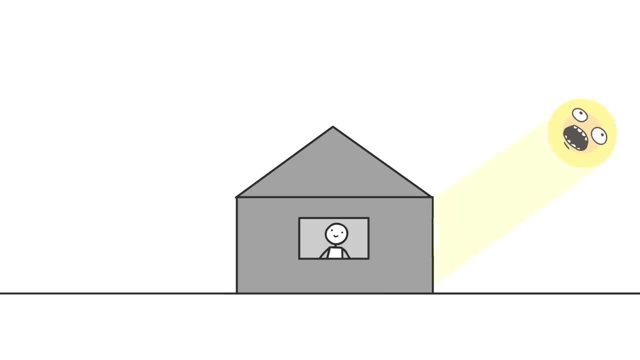 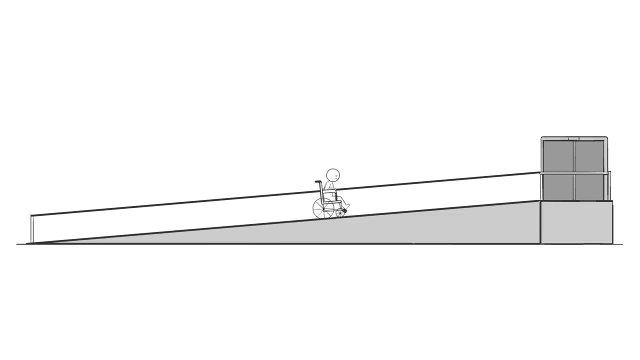 Mattress and a cold terus the same. The ground and the ceiling are all matte and these are hanging on the top Into the ceiling, continue to be a little wavy, although most of the surfaces are knee deep, Slightly looking downer. the stairs and ramps are an absolute forbidden condition. 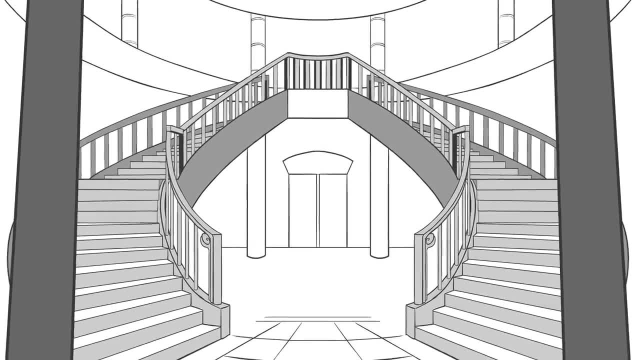 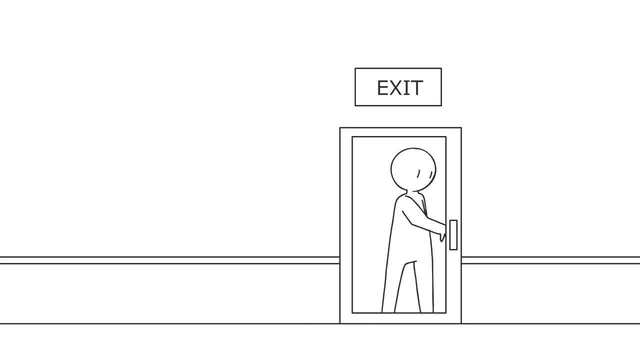 Symetry is cursed. You don't really need double staircases that both lead to such a location. I feel like people really only use these for prom photos. And finally, or at least this is all I can think of right now, all exit doors should.